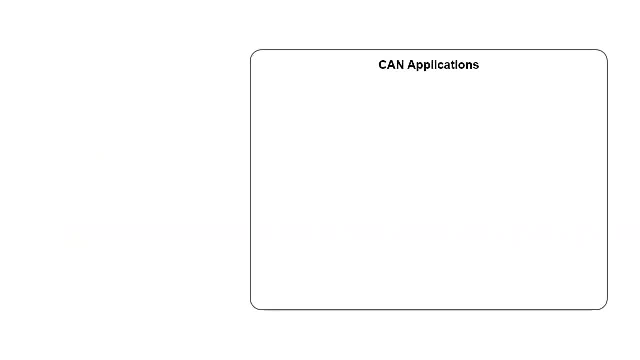 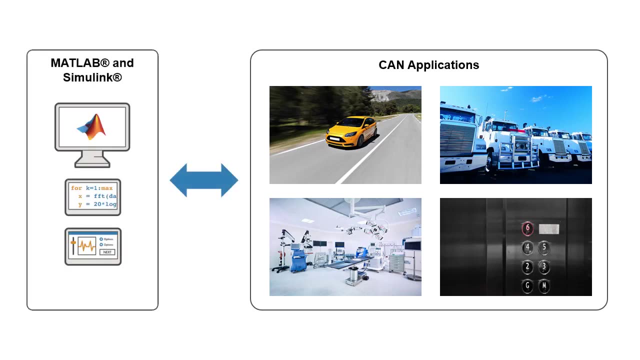 Nowadays, you can find CANbus used in a variety of applications such as passenger vehicles, heavy trucks, medical equipment and elevators. MATLAB, Simulink and Vehicle Network Toolbox provide functions, blocks and apps to interface with and retrieve data from CANbuses. 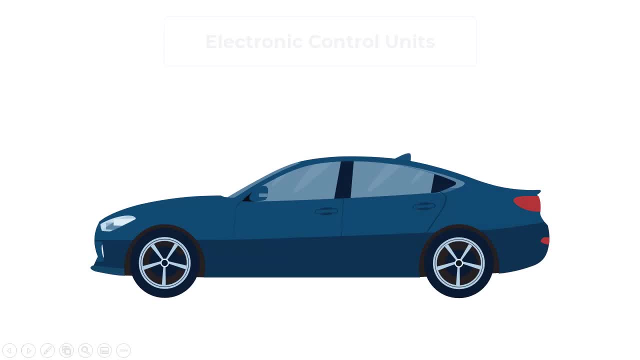 CANbus is the system that connects nodes and electronic control units, or ECUs, in a vehicle network system. The CANbus provides a low-level interface that allows CANbuses to communicate with each other. It's easy to use to communicate directly with each other through a simple serial bus. 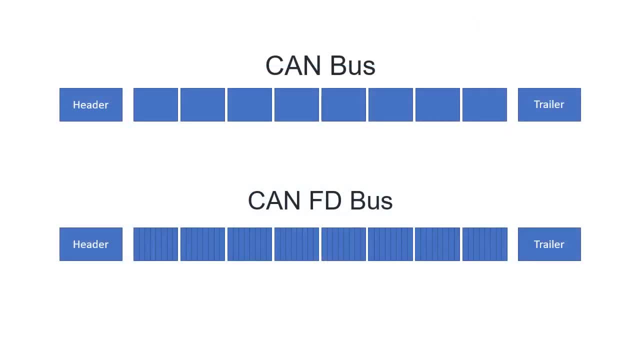 CANfd or Controller Area Network. Flexible Data Rate is a protocol that builds upon CAN. The main difference between CAN and CANfd is that Flexible Data Rate in CANfd allows for higher data throughput on the bus. For comparison, the maximum CAN frame size is 8 bytes, while the maximum CANfd frame size is 64 bytes. 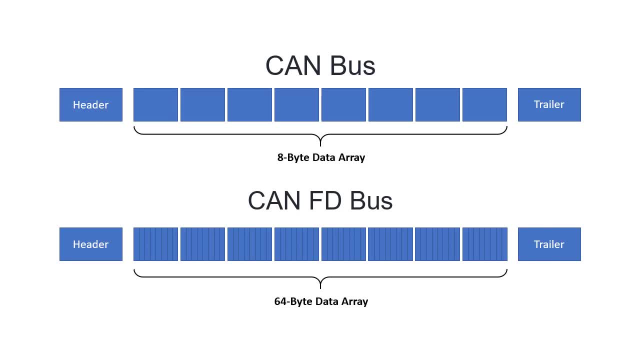 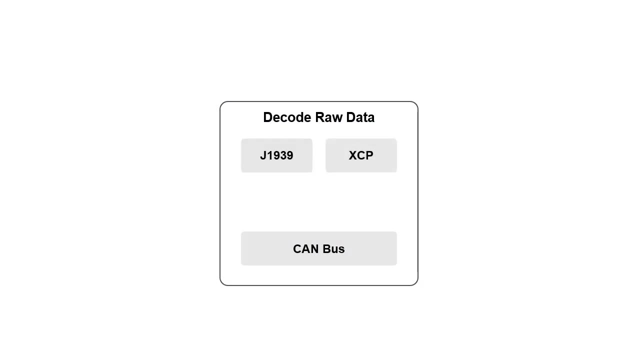 CAN and CANfd are advantageous because of their low-cost, decentralized network, system efficiency and node flexibility. Higher-level protocols such as J1939, or XCP define communication systems on top of the CANbus that define operations for specific applications, such as heavy vehicles for J1939 and vehicle calibration for XCP. 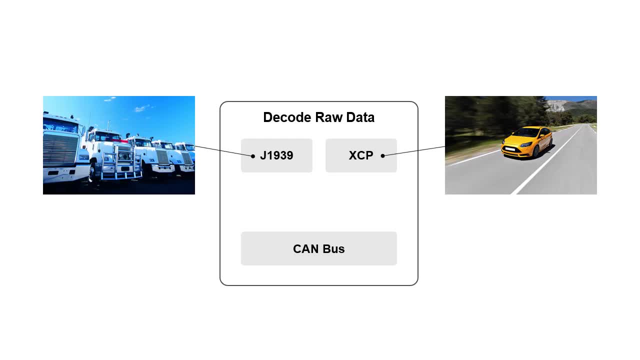 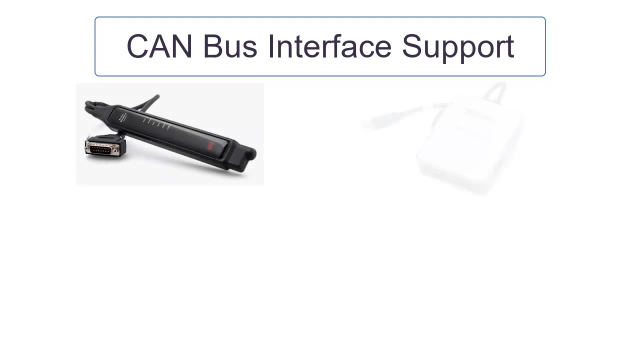 Raw data from a CANbus can be extracted and decoded into protocol-specific information using a CAN database file or DBC. MATLAB and Simulink support CANbus interfaces from manufacturers such as Kvaser, National Instruments, Peak System and Vector. 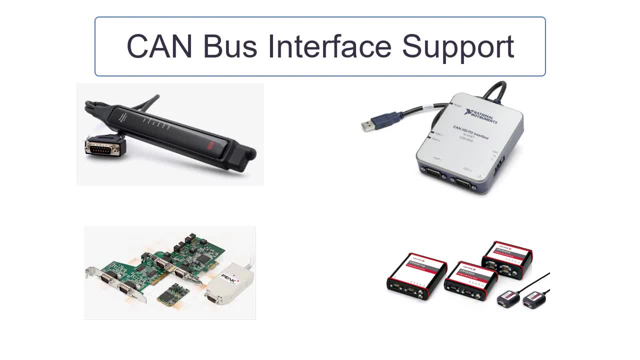 Vehicle Network Toolbox supports CANbus interfaces that connect directly to your PC via USB, PCI and USB. Vehicle Network Toolbox supports CANbus interfaces that connect directly to your PC via USB, PCI and USB. Vehicle Network Toolbox supports CANbus interfaces that connect directly to your PC via USB, PCI and USB. 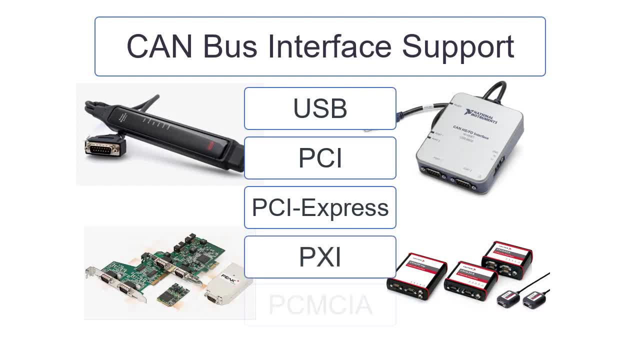 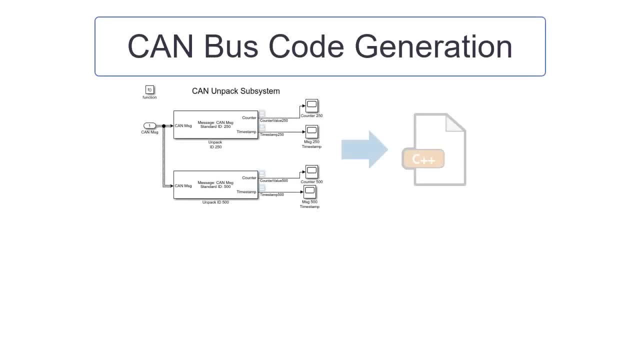 PCI Express, PXI and PCM-CIA. PCI Express, PXI and PCM-CIA Vehicle Network Toolbox provides Simulink blocks for generating C or C++ code from your CANbus workflow. Certain blocks, such as CAN and CANfd, Pack and Unpack, support code generation for embedded targets.